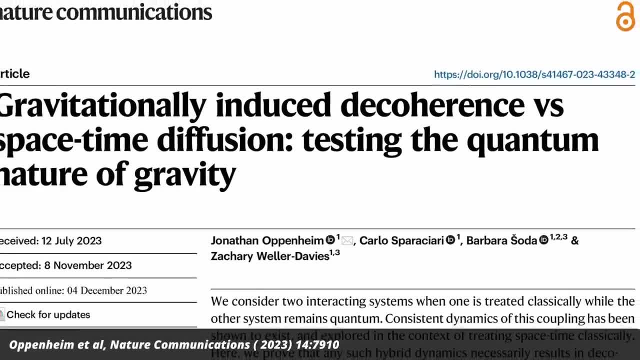 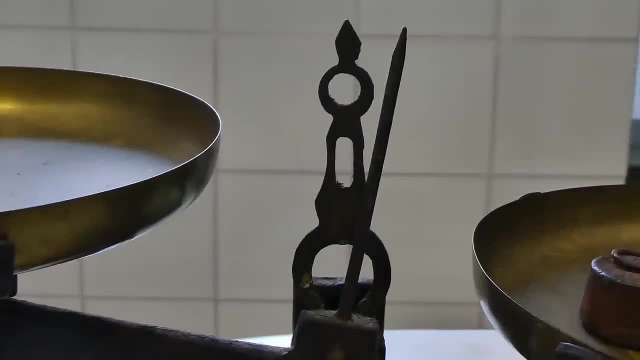 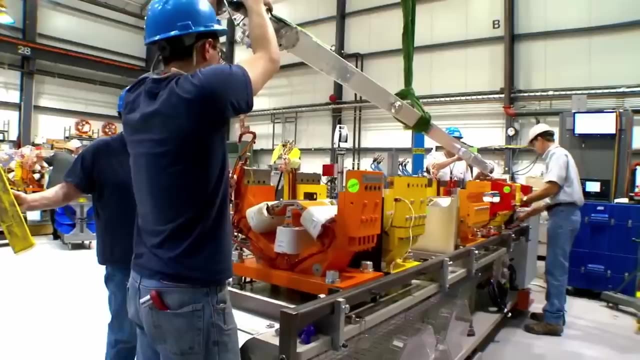 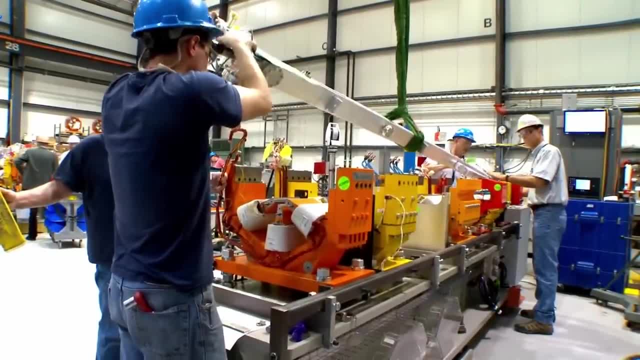 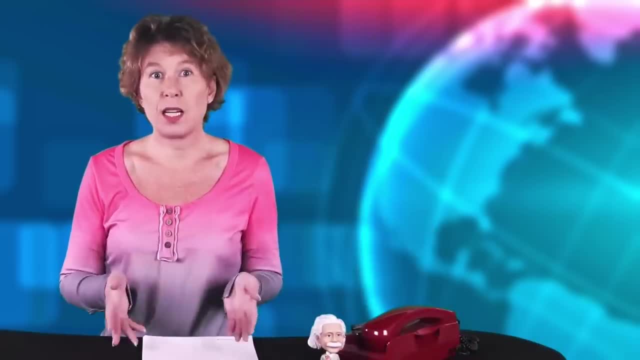 Tabletop experiments are what physicists call an experiment that doesn't cost billions of dollars. Like you know, particle colliders. Another interesting thing about this idea is that it has a collapse of the wave function built in, so the measurement problem of quantum mechanics disappears. 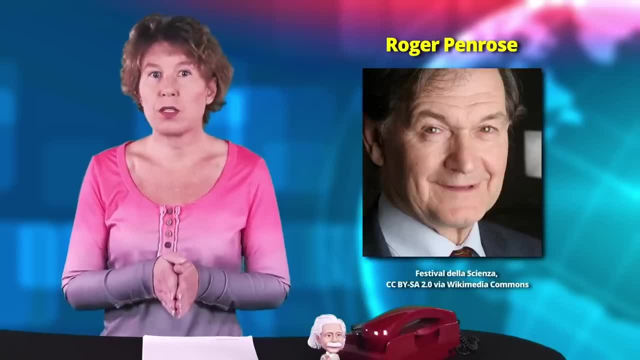 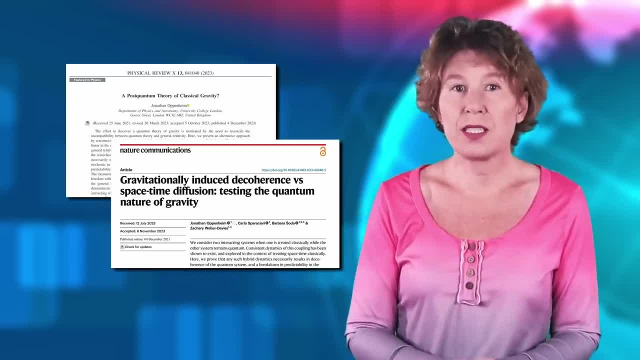 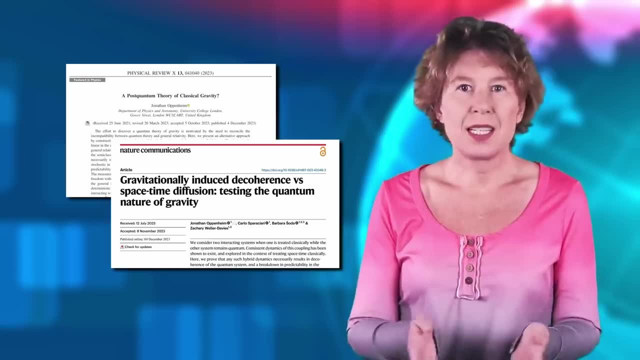 And Roger Penrose that gravity is what causes the collapse of the wave function. But Oppenheim's work is a mathematically more complete treatment and indeed I find it quite impressive. It'll take me some time to fully digest the paper, so let me just say this is a very 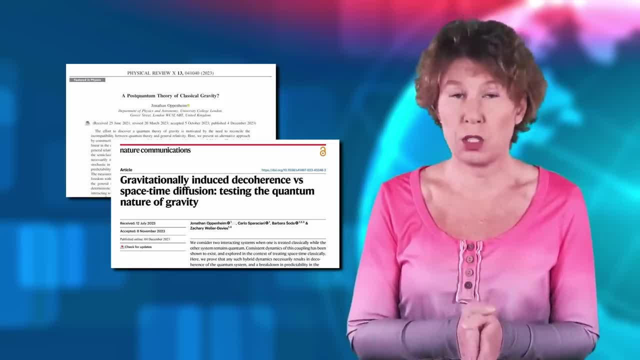 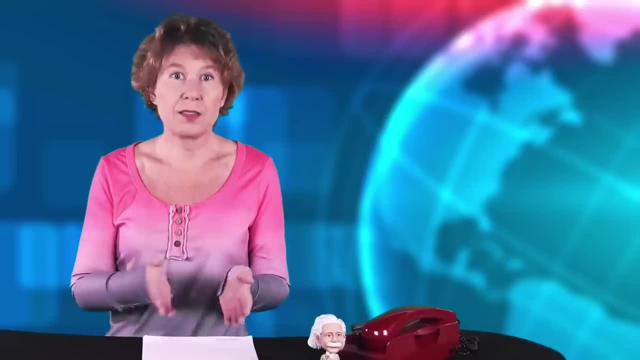 strong contender that I think can plausibly claim to solve the problem. However, there are always multiple ways to solve mathematical inconsistencies like that between general relativity and quantum mechanics, relativity and quantum mechanics, And this is only one of them. So in the end experiment. 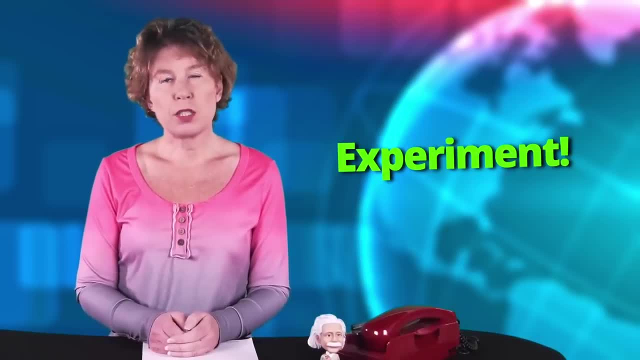 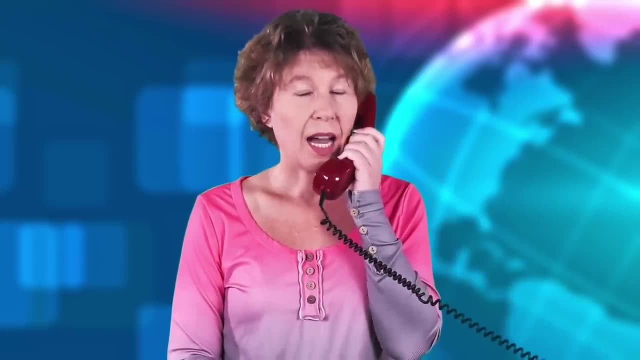 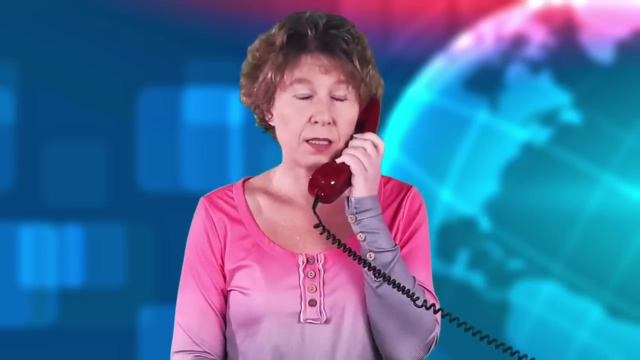 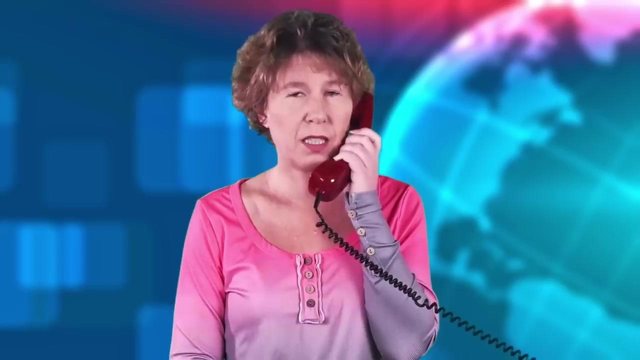 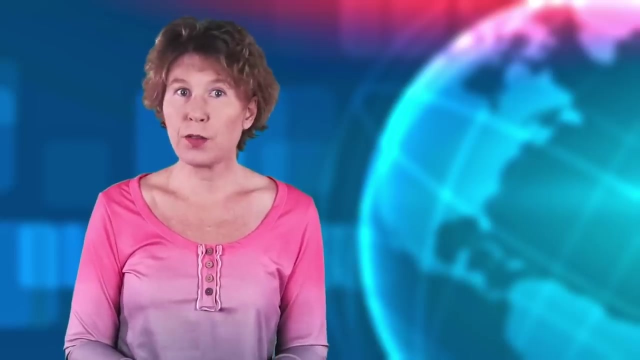 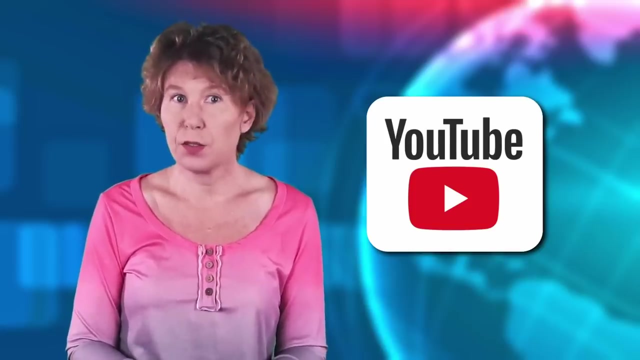 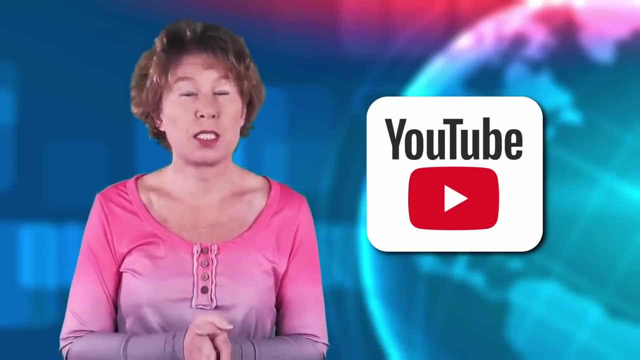 must decide. I wonder what Einstein would have said about this. Hello, Hi Albert. Yes, I'm afraid that means that God is still playing dice. Oh, I didn't know that. craps is a dice game. That explains a lot. Well, thanks for calling in. Bye.